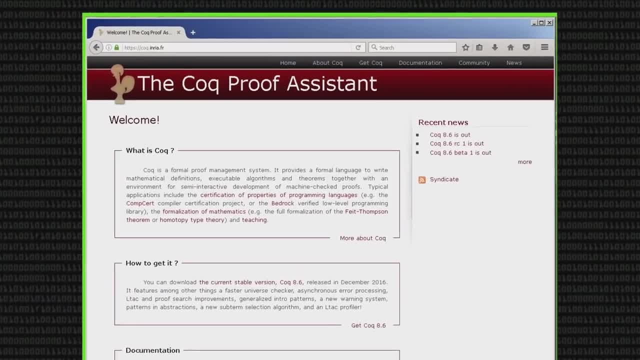 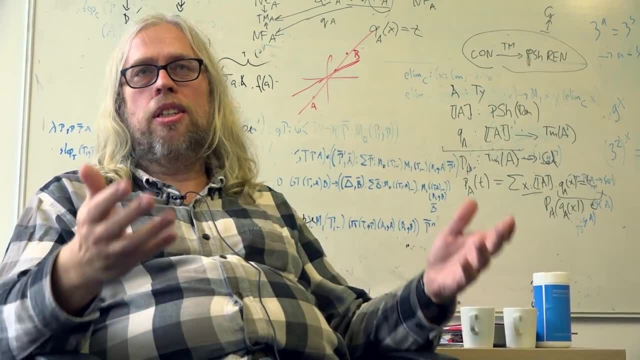 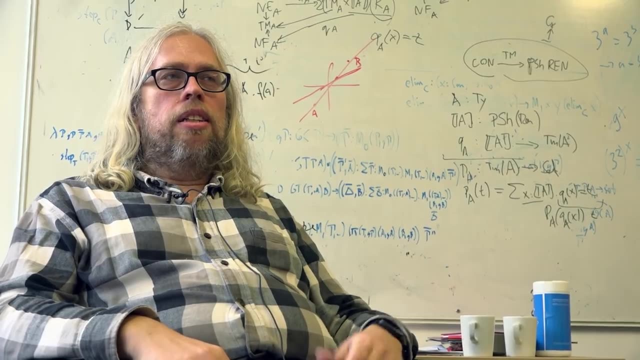 It's a French system, I think they called it a bit to upset English speakers. We could just do mathematics, as has been done, using something called set theory. Many people learn about sets and elements and this sort of thing And just formalize this. 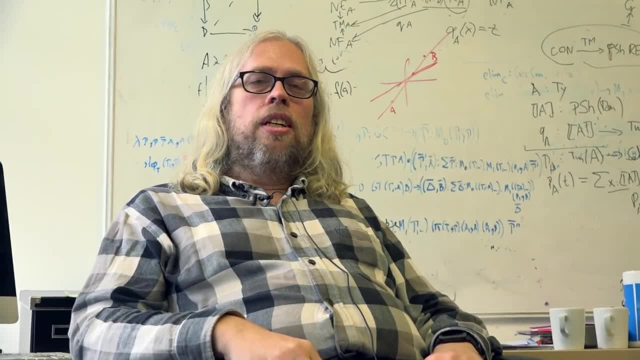 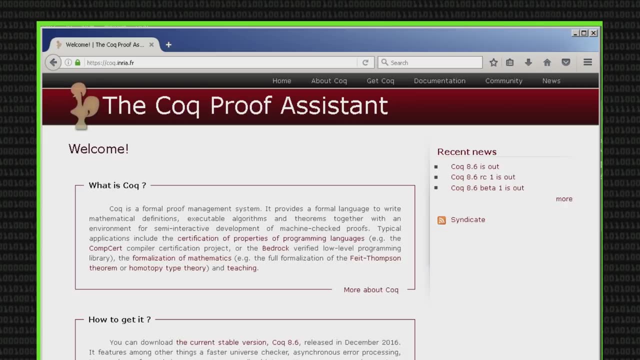 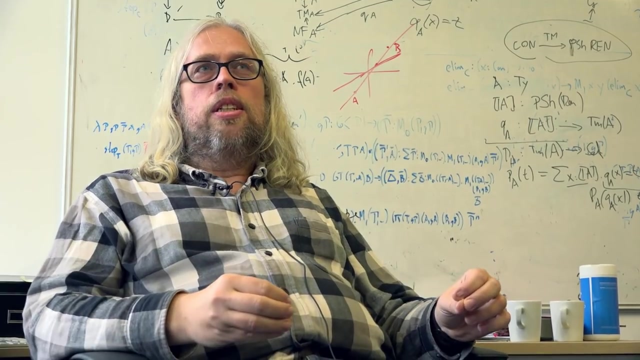 But I think if we would do this, we really miss an opportunity. This Coq system, for example, is actually based on a programming language. It's a programming language called type theory. So this type theory is at the same time a programming language. 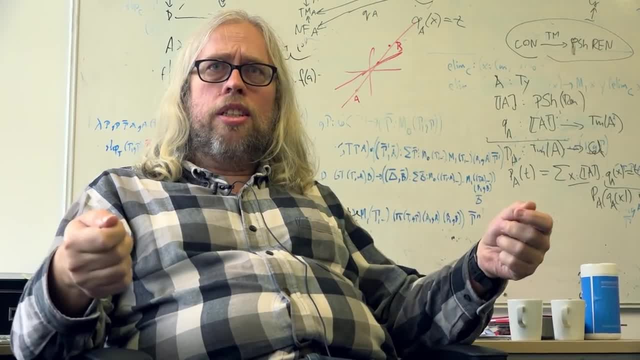 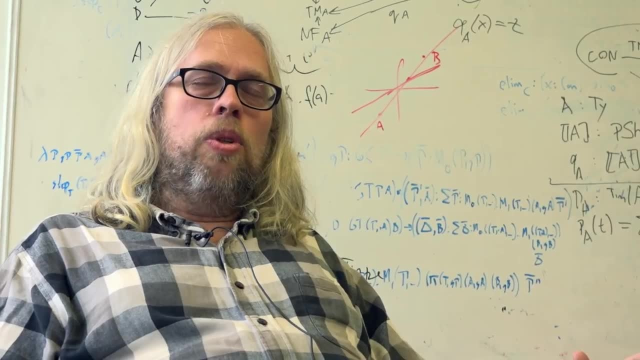 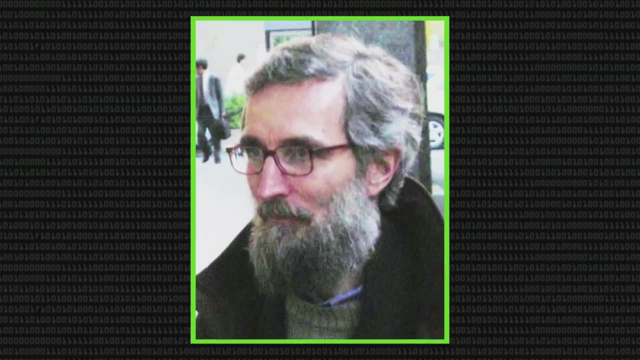 And it's a logic so you can do logical reasoning, And it's a replacement for this language mathematicians use, called set theory. It's a more recent development going back to the 70s. A Swedish mathematician and philosopher, Per Martin Löf, 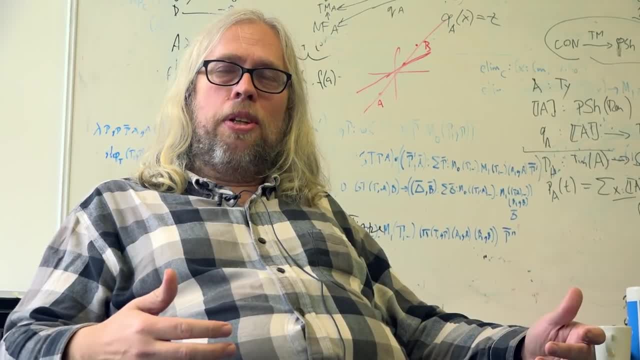 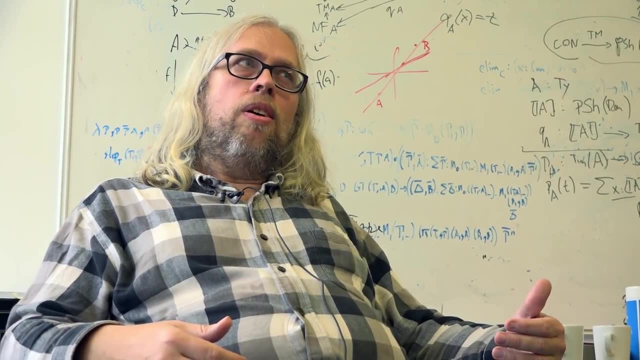 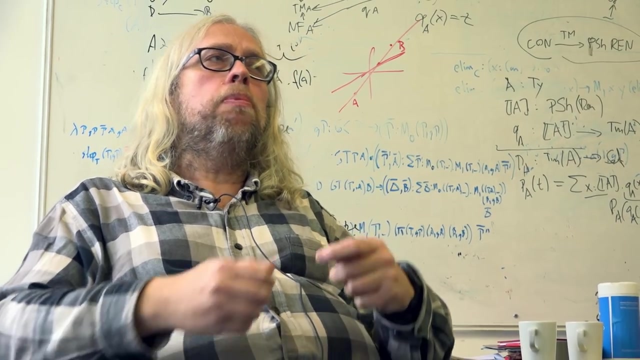 he wanted to capture what was called constructive mathematics. By constructive mathematics we mean that we can actually always obtain a result That we don't just claim. For example, if you have a function, you may have no way to calculate the answer. 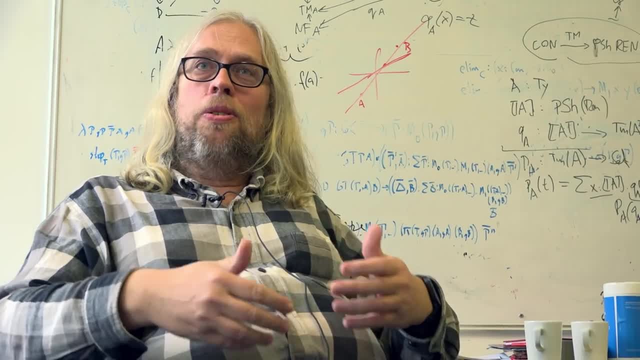 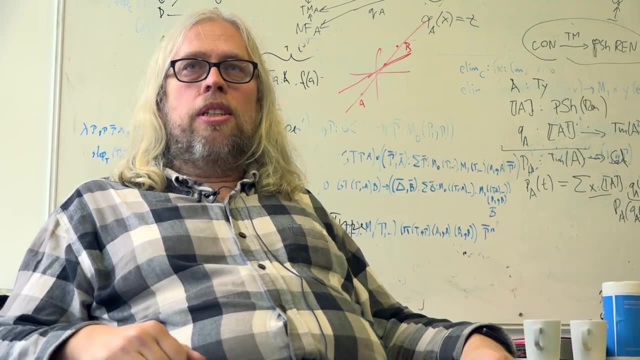 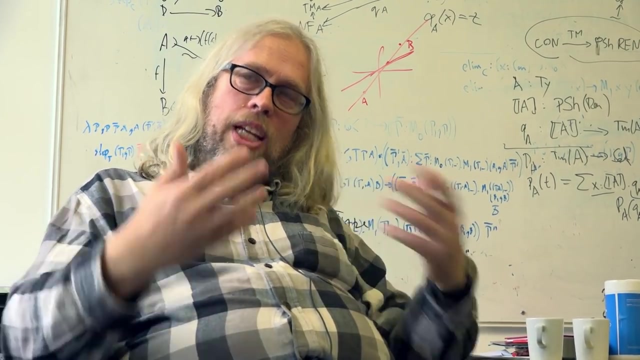 In constructive mathematics there's always a way to obtain an answer. If you say there exists a number with some property, in classical mathematics you may not know the number. In constructive mathematics you can only make this claim if you can actually provide a number, a concrete number. 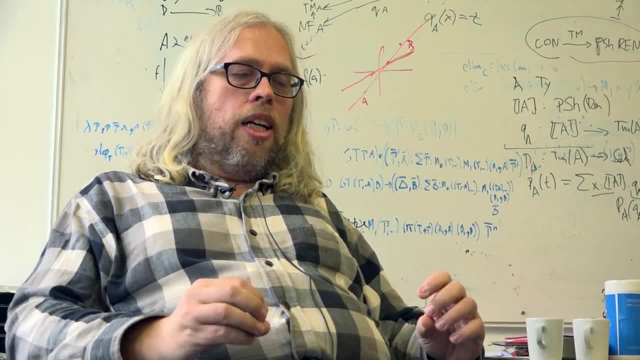 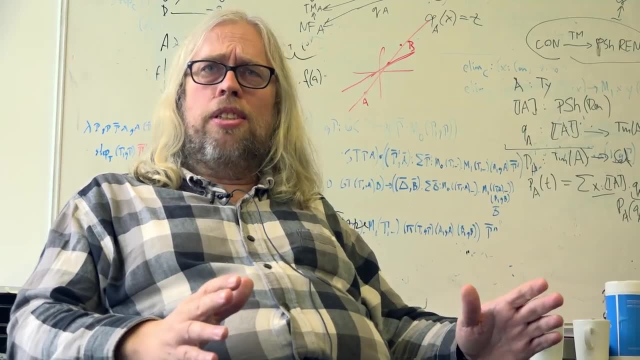 So, And Per Martin Löf? he had nothing to do with computer science. I mean, he was really a philosopher, a mathematician, a very interesting guy. But then people thought, OK, this idea of always, you get an answer. 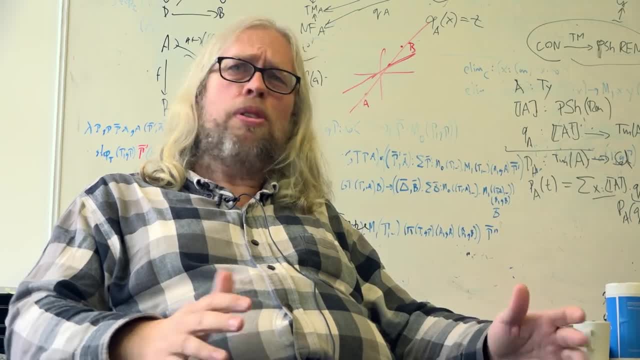 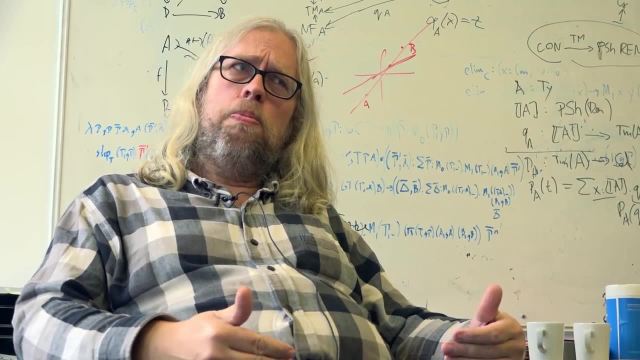 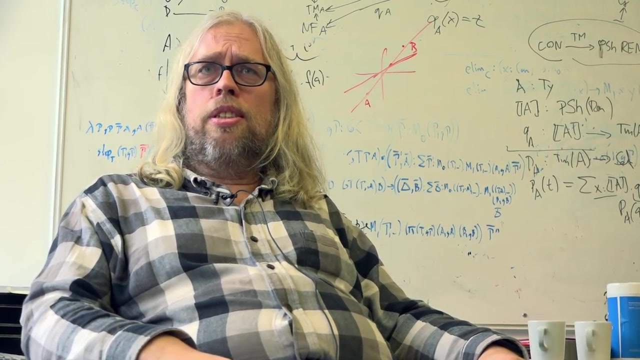 doesn't this correspond to like writing a computer? He said, yeah, yeah, sort of, It's like a computer program And this has been made more precise and has been used. So people started basically to write, implementing on a computer this type theory. 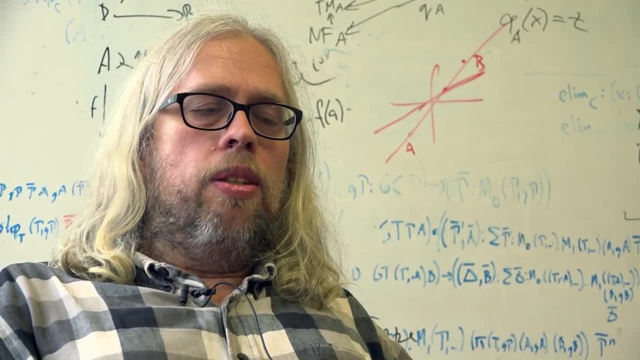 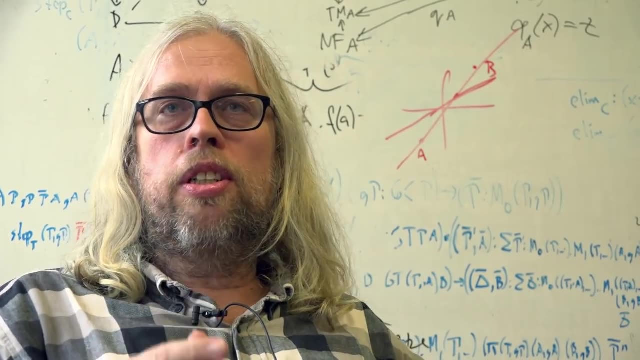 Type theory uses the types we have in programming languages. So type like, for example, the type of booleans, the type of integers or the type of functions from integers to booleans. so input is an integer, output is a boolean. 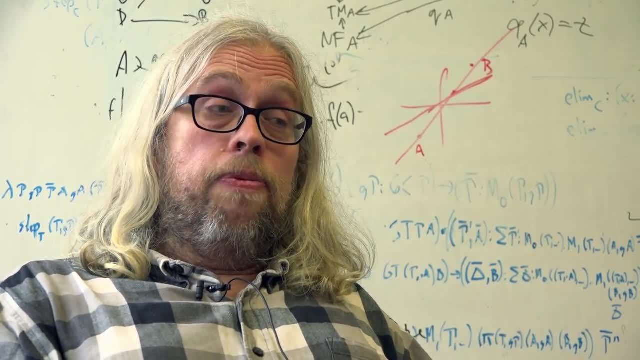 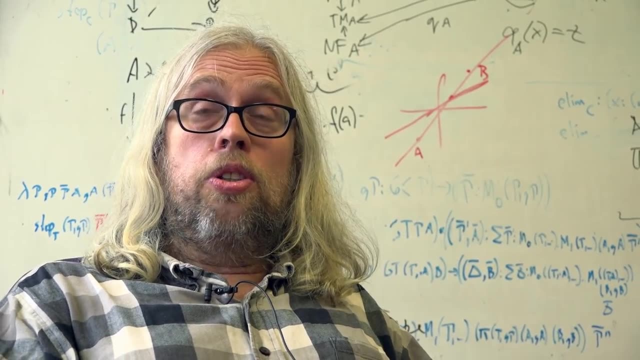 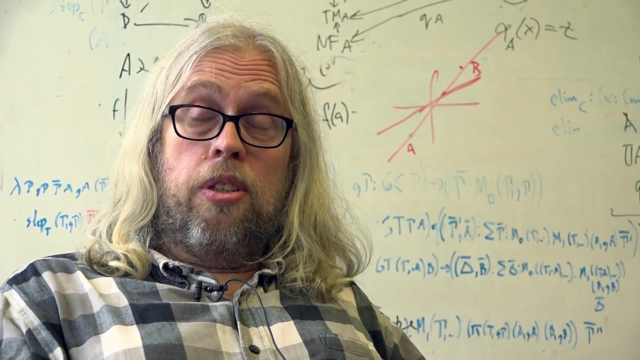 and so on. So these are types, And a very important observation is that we can use types also to model logical reasoning, to model logical propositions. So if you have a proposition, an expression in the logic I mean, for example, there are infinitely many prime numbers. 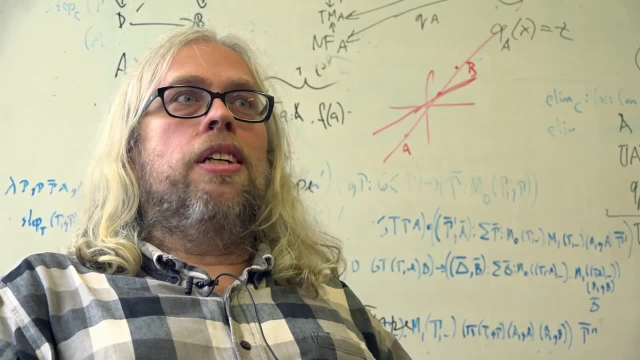 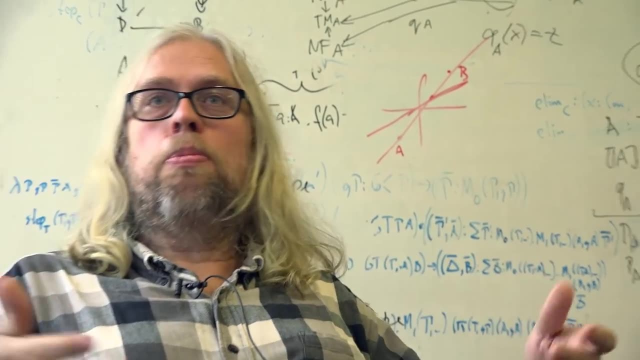 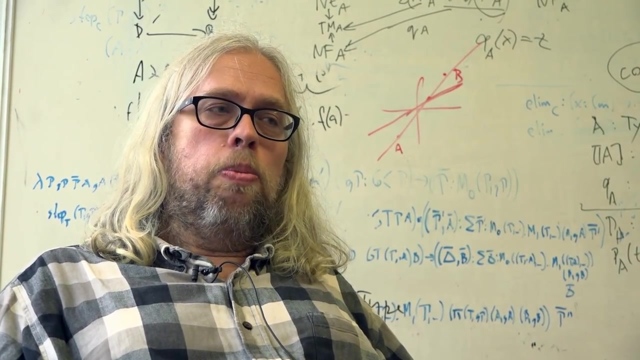 as a proposition, or every two numbers, natural numbers. one is less than the other, or they're equal, or one is greater than the other. These are propositions, And the observation is that we can, for every proposition we can, associate a type. 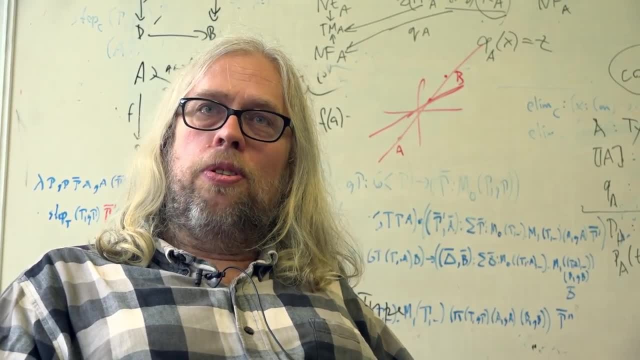 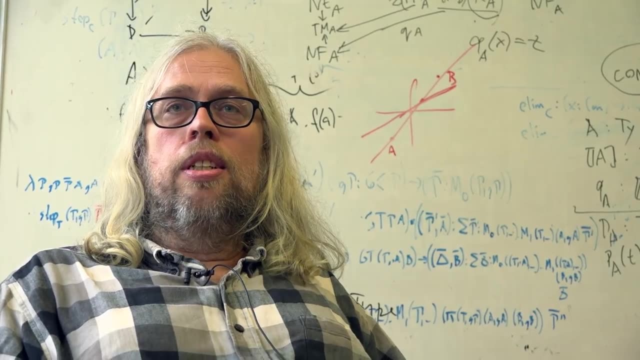 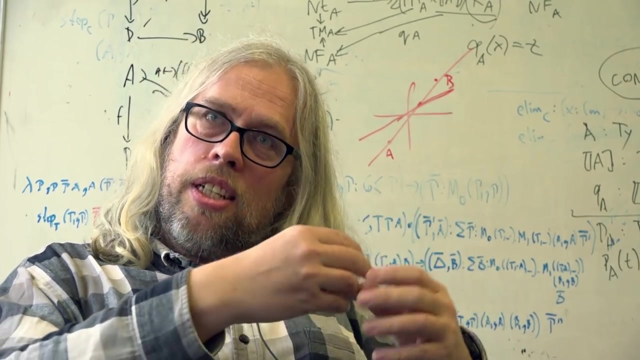 And that's the type of evidence or proof for this proposition. This is called the Curry-Howard equivalence. So whenever you have a proposition you find a type such. if there is a program of this type, then you know this proposition holds. 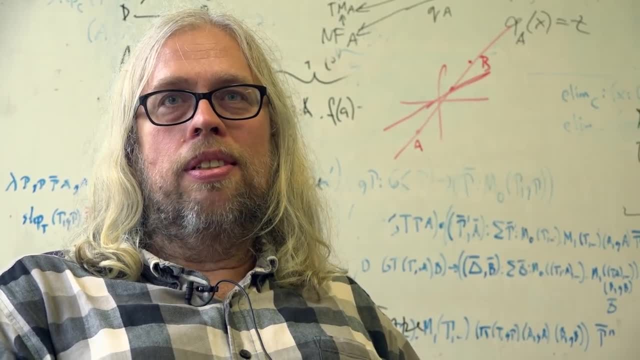 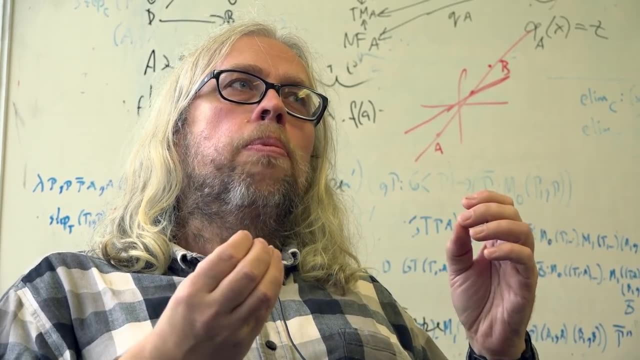 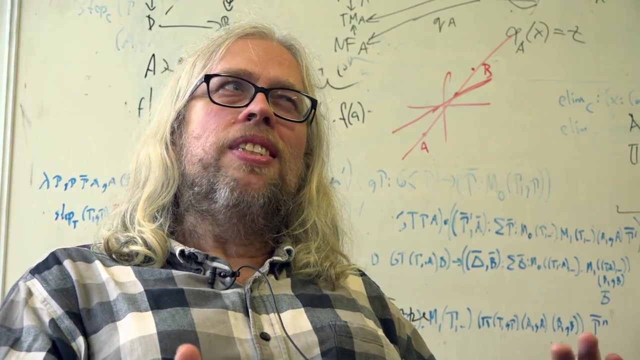 So this is computing getting its elbows in and getting stuck into some mathematics. Yes, And I would say, OK, there is a using type theory. it's very natural to do it on a computer, whereas set theory seems to be rather alien. 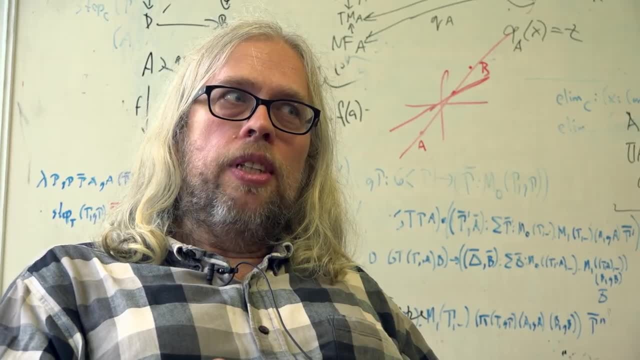 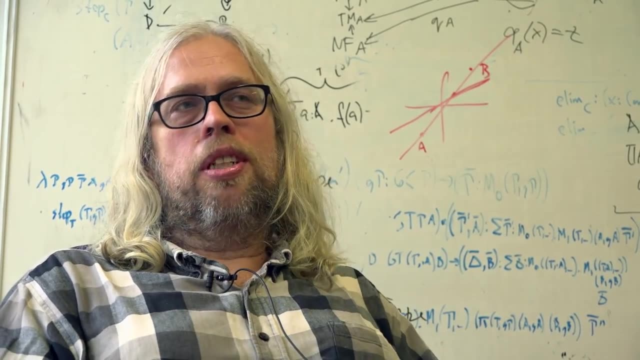 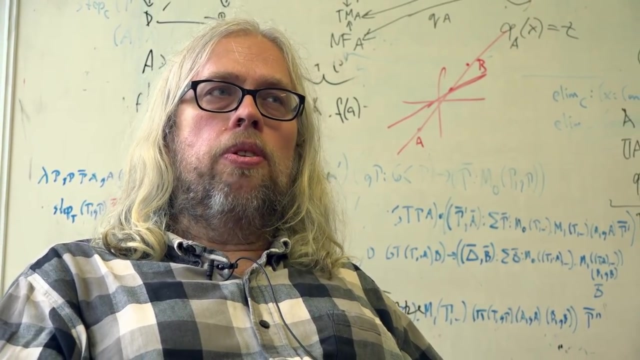 to using computers. In set theory, for example, there's also the notion of a function, but it's a derived concept. You see, you have a set of pairs which have certain properties. There's not this idea like in type theory. 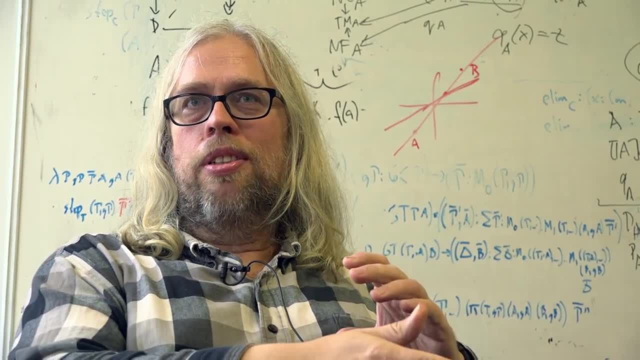 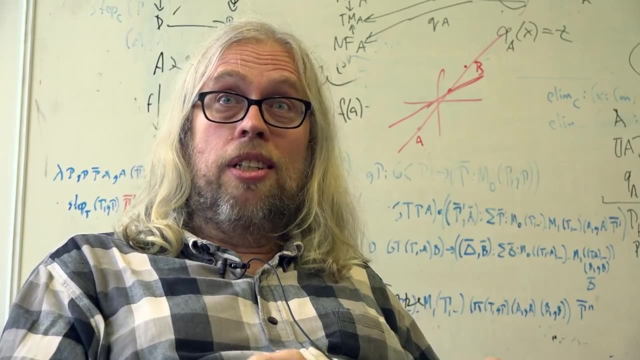 that a function is something where you put something in and you get something out which comes from computer science Or which corresponds to how we think in computer science. So a function in type theory is something you can actually compute with, Whereas a function in mathematics. 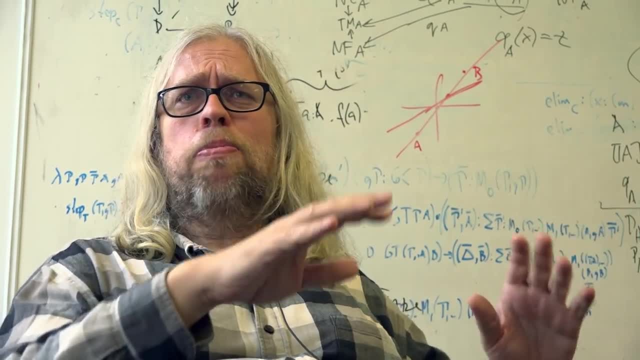 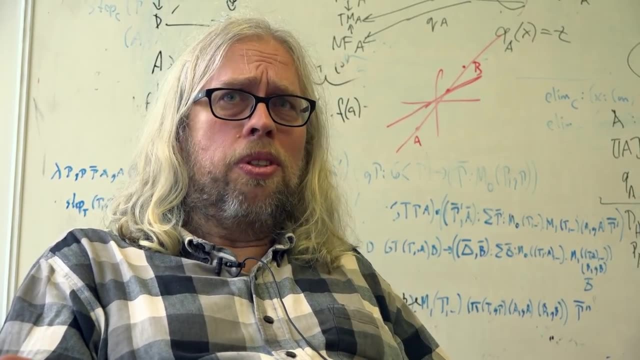 and in set theory is something like just a set of pairs of all the possible inputs with corresponding outputs. But a function in mathematics may be something you cannot compute. So I'm always saying this is not a good name, then call it a function. 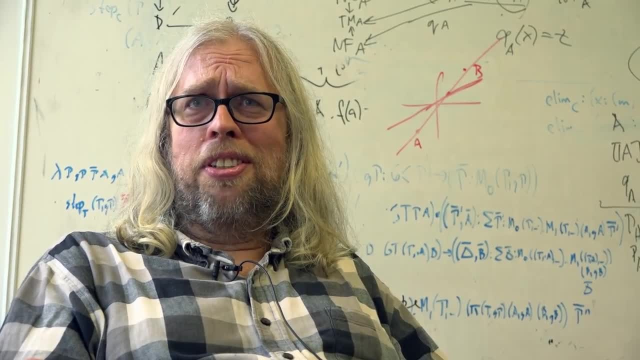 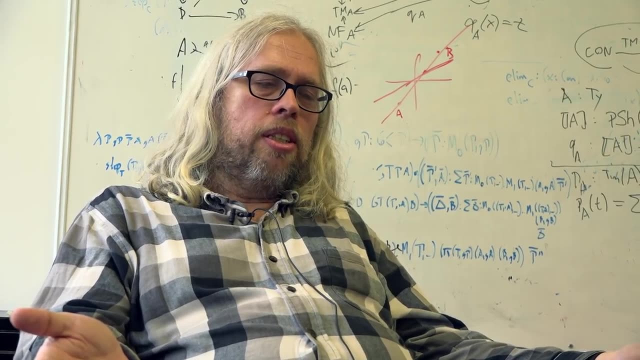 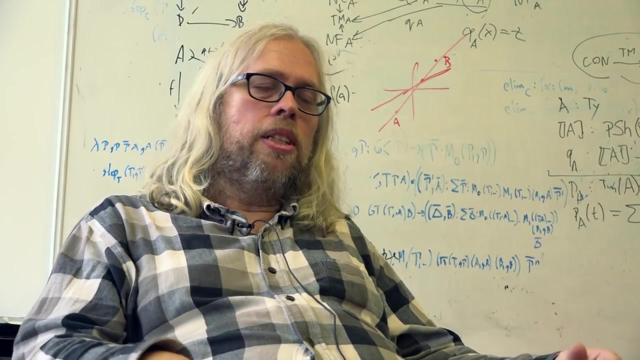 because a function which doesn't function shouldn't be called a function. It's a dysfunctional function. Yeah, a dysfunctional function. Type theory has got some other interesting features which have been discovered or made explicit more recently, And this is work which was started. 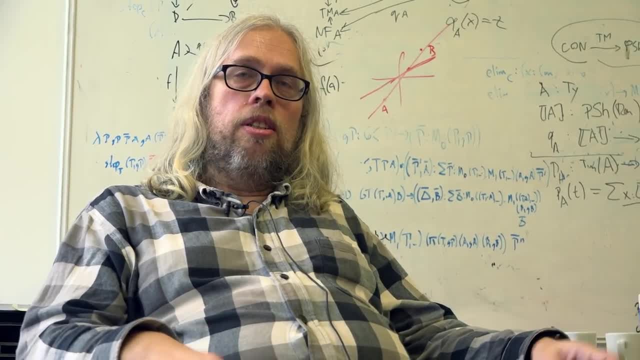 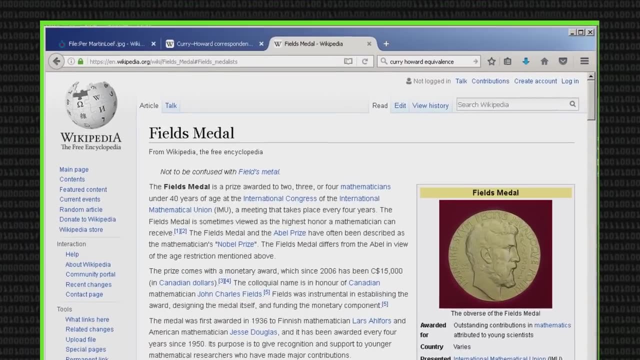 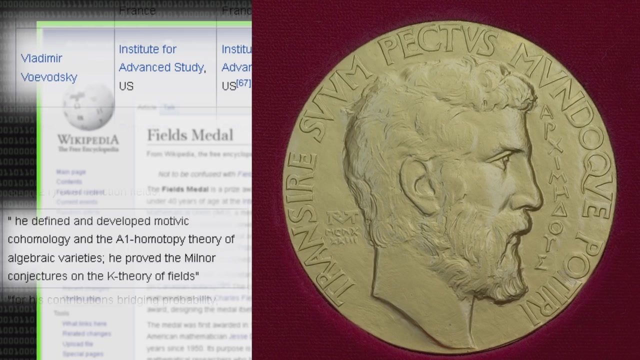 by a mathematician. actually, He's called Vladimir Vovotsky and he's a field medalist at the Institute for Advanced Study at Princeton. He's doing something called homotopy theory. So homotopy theory is a quite abstract area of mathematics. 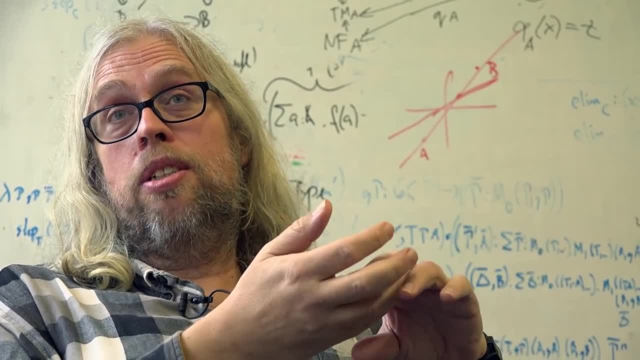 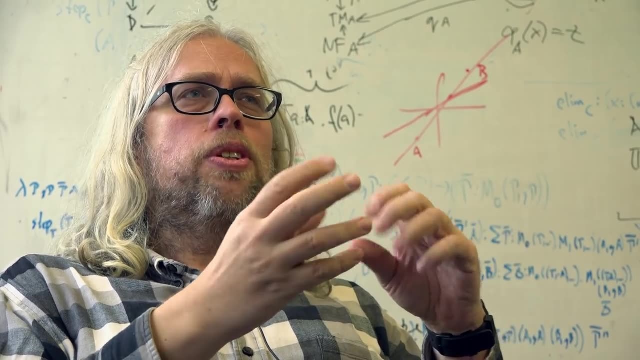 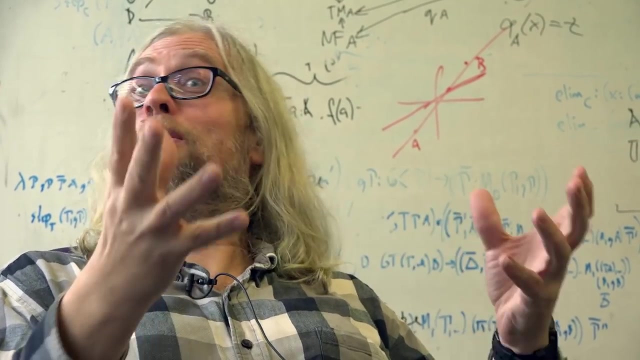 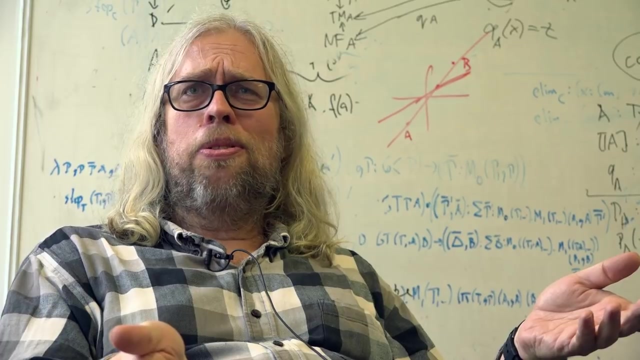 where you try to understand some geometric object, very abstract geometric objects, And you really identify geometric objects which you can transform, like plastic or Play-Doh, which you can transform one into the other in continuous transformation And first of all that doesn't seem to be anything to do. 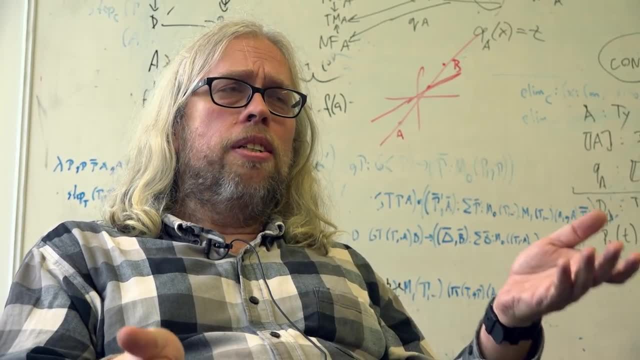 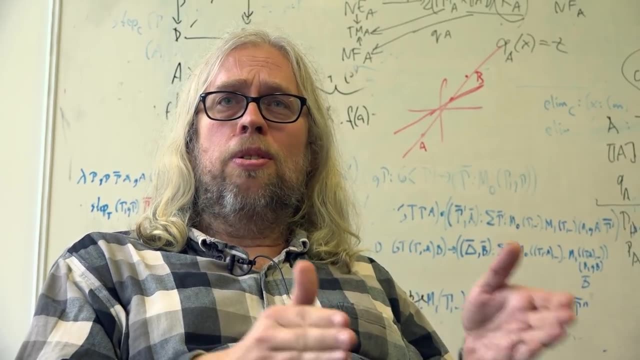 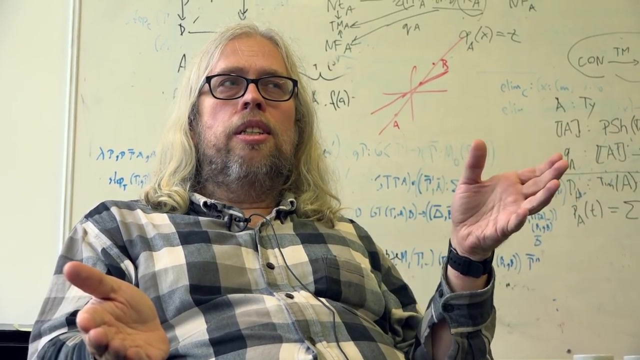 with this type theory I mentioned. But Vladimir Vovotsky observed that actually there's a close connection between type theory and homotopy theory, which leads to this new idea which is called homotopy type theory, And so the idea here is that when in type theory 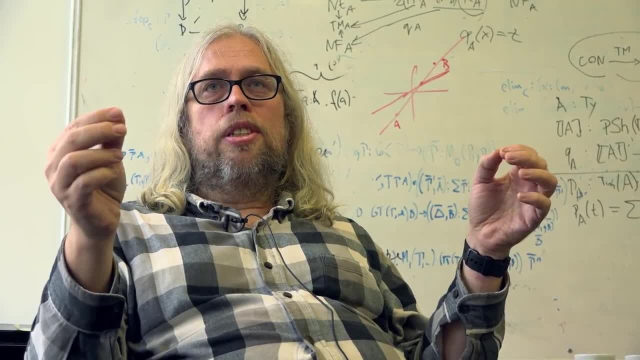 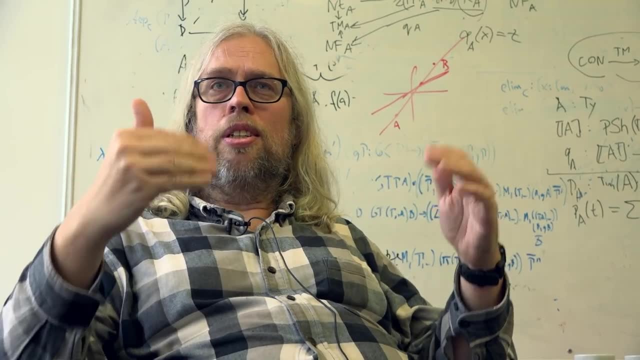 you prove that two things are equal. this is like having one of these surfaces and having a path. You have a path between these things And then you can also ask yourself: are two equalities equal? So we have sort of a path between paths. 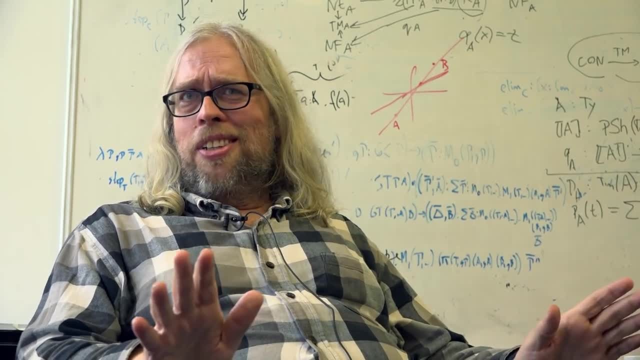 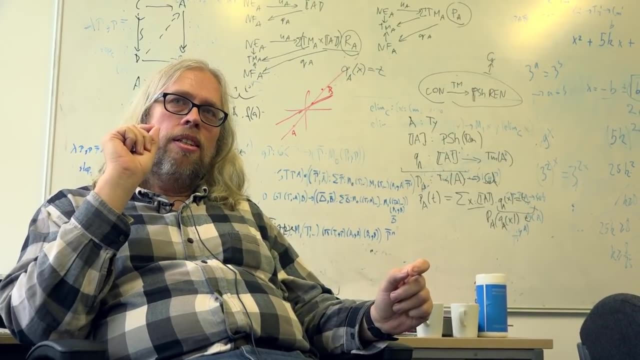 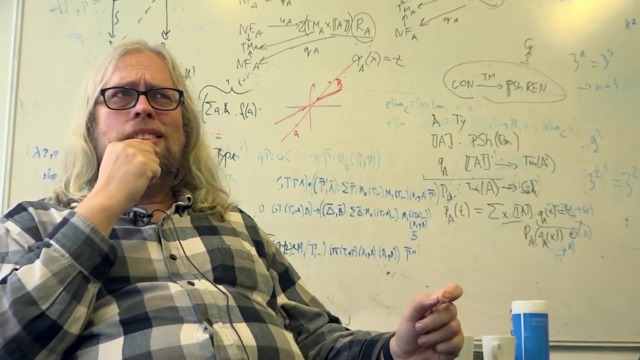 a continuous transformation of paths. Okay, It's getting quite abstract. now It's getting very abstract. Are these Play-Doh objects a bit like a kind of way of visualizing these ideas, Or is that what he's discovered? No, it's not really. 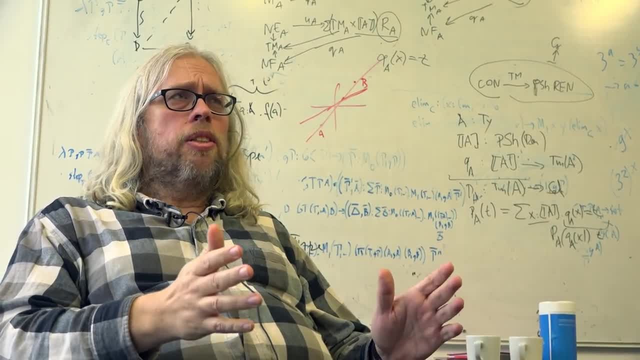 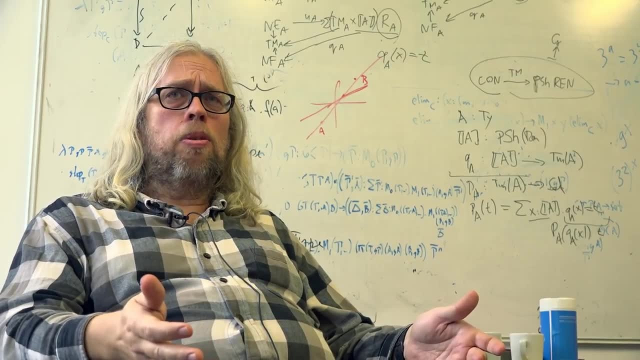 It's rather surprising because we start with something which I call type theory, which is a programming language and it's a logic, as I have explained, And then there is this homotopy theory, which has completely different roots in what's called algebraic topology, which is like I mean. 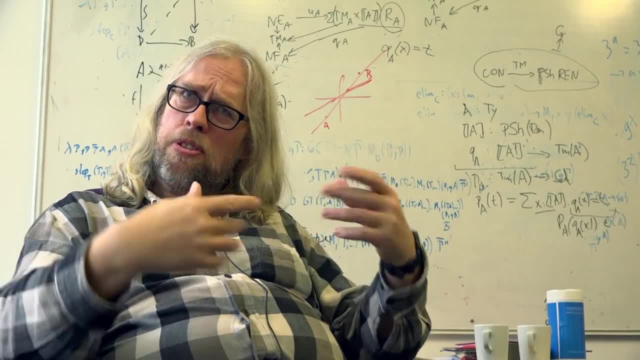 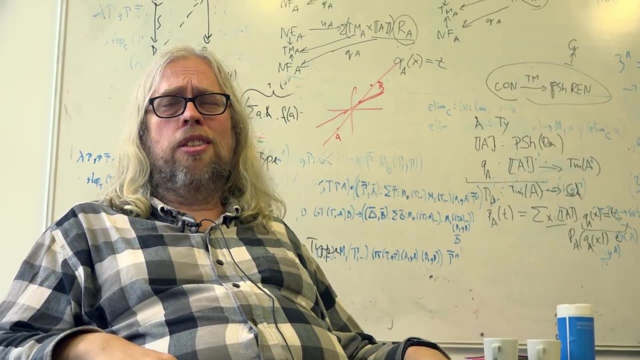 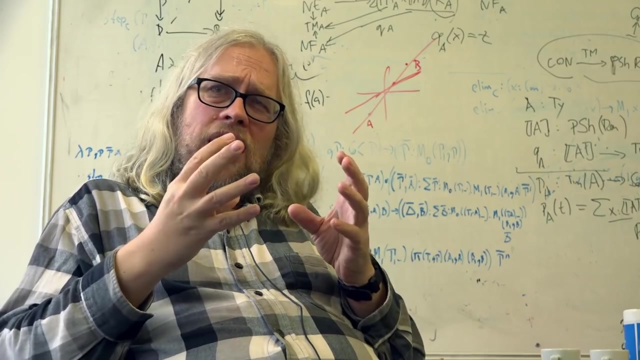 topology is the idea of describing continuous phenomena like real numbers and surfaces and so on, which are important in physics and so on. And then in homotopy theory, people did it more and more abstractly. They tried to distill the essence of these objects. 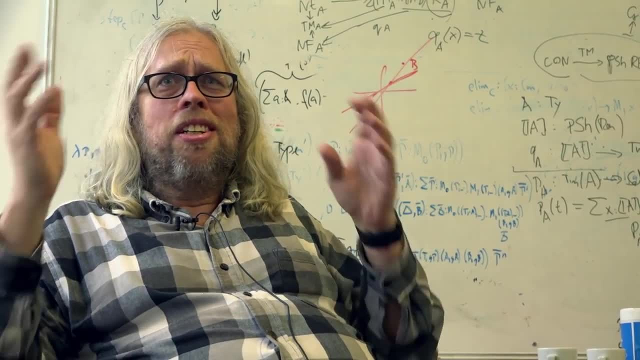 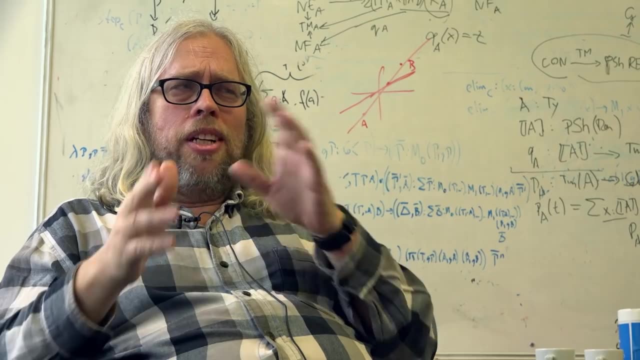 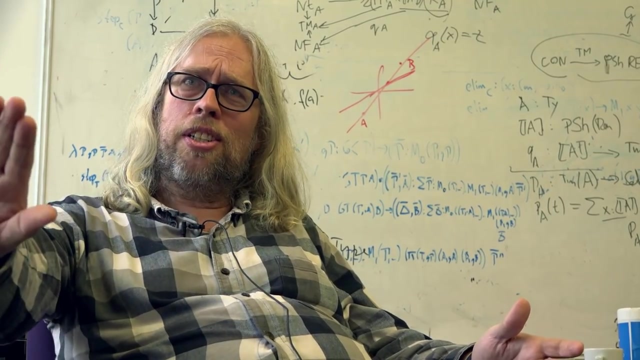 They are infinitely dimensional. no, really good intuition for what's going on. But then the surprising thing- and this is one of the surprising reuses of mathematics- that you go completely abstract in one direction and you come out somewhere completely different. Yeah, 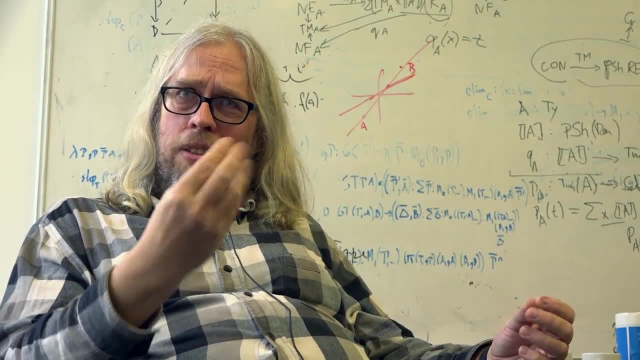 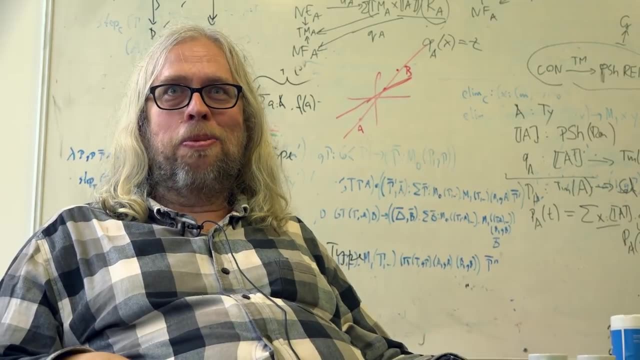 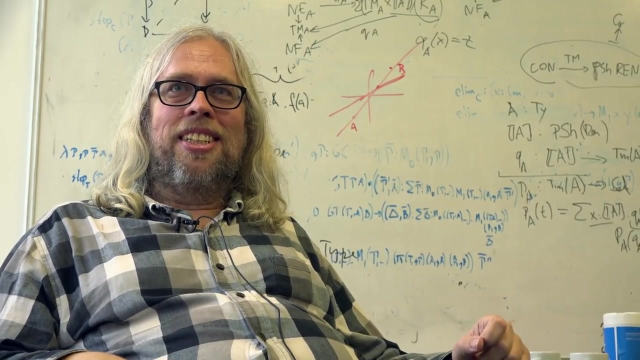 And this is the relation between type theory and homotopy theory. Okay, So it's not very direct. It's not like we have a type and then we have a picture which corresponds to this type. It's not like this, It's much more indirect. 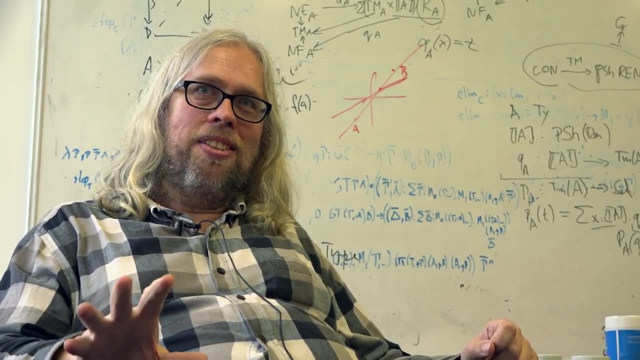 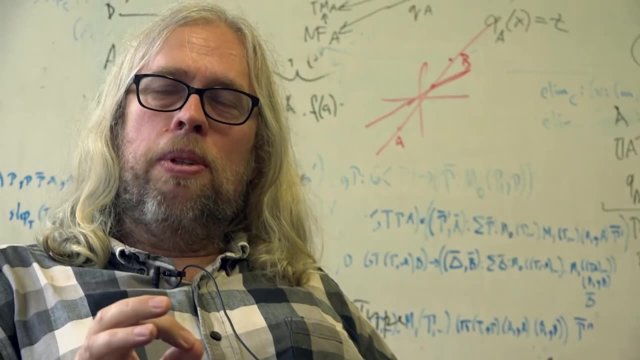 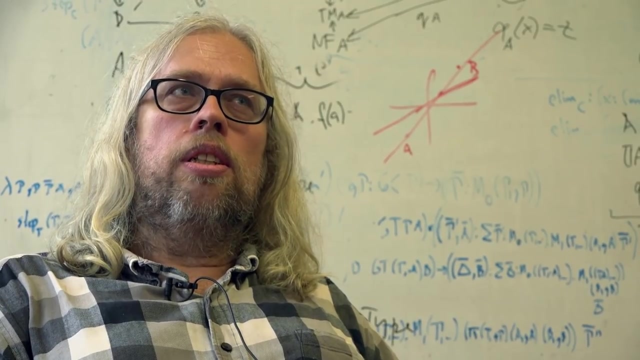 But the mathematical principles underlying this homotopy theory and type theory- they match up surprisingly well. Maybe a good question is: what is the payoff? I mean, what does this buy us? And I think there are some very exciting opportunities now where type theory shows. 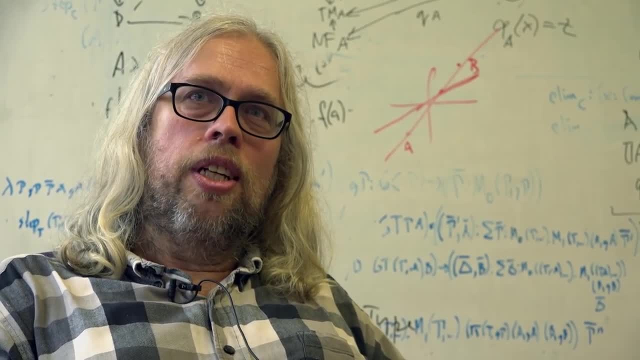 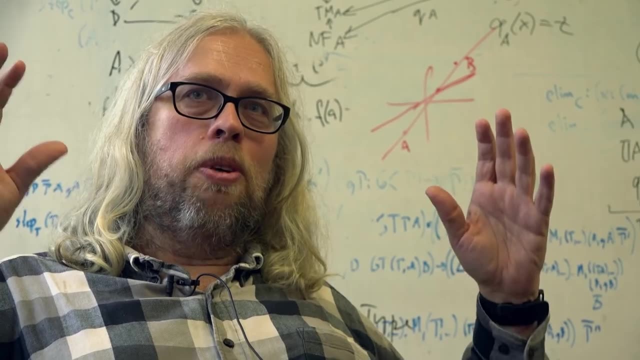 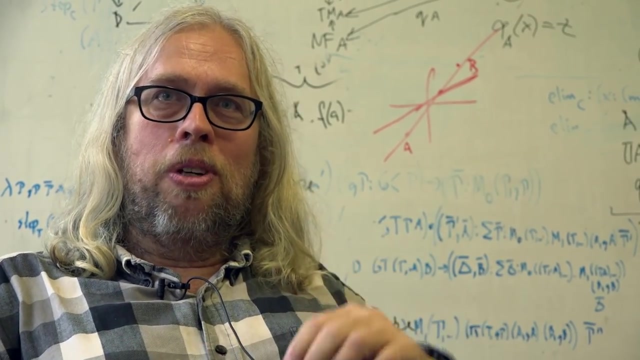 its superiority over set theory, And this has to do with abstraction. If you want to build large mathematical libraries, you have to climb a ladder of abstract reasoning. You don't want to do everything on a very concrete level, You have to do things abstractly. 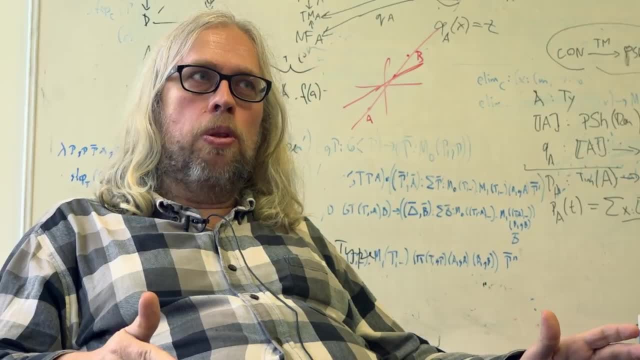 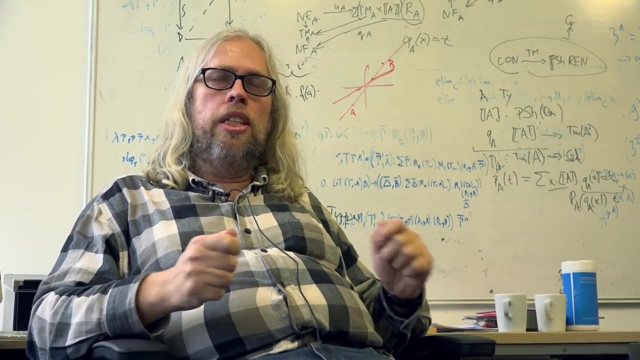 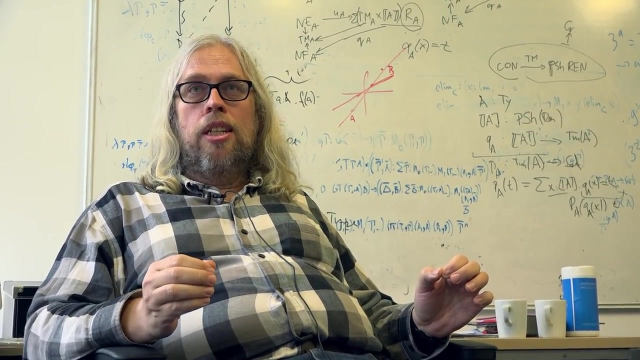 That's the power of mathematics. Type theory, and especially homotopy type theory, in its very structure is designed in a way that you cannot talk about the details of how things are actually implemented. So example: natural numbers In set theory. 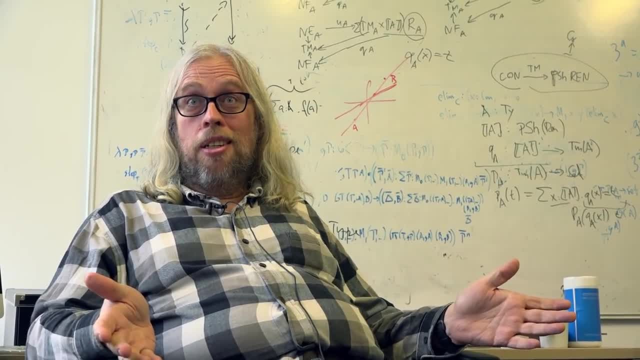 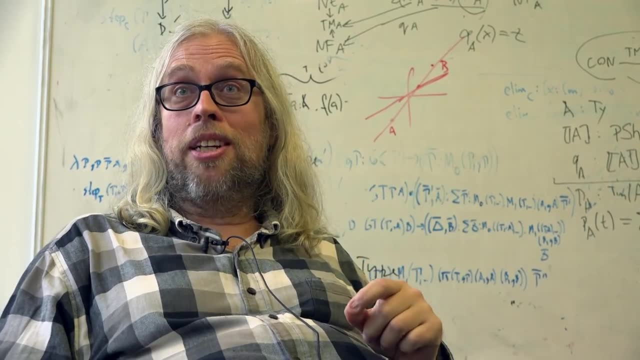 natural numbers are sets. That may be surprising, But in set theory, everything is a set And there's a particular encoding of natural numbers using sets, using these curly brackets. Well, there's more than one, So you can use sets to encode natural numbers. 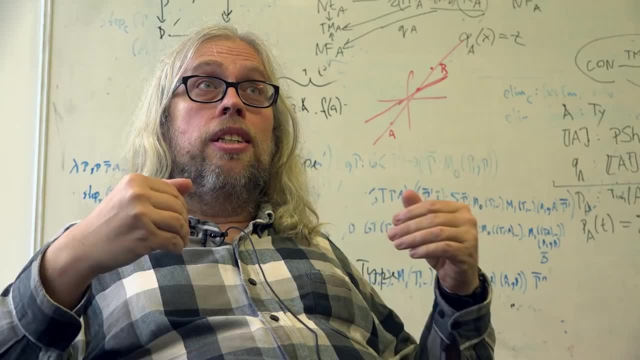 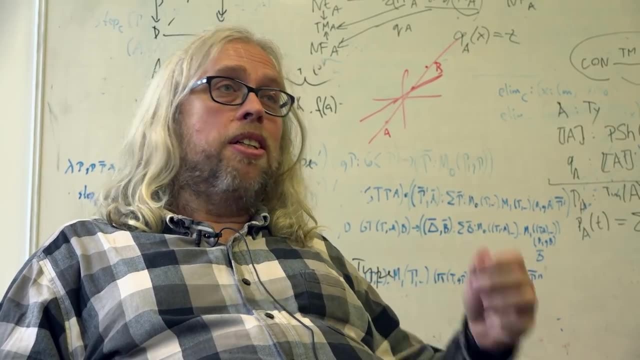 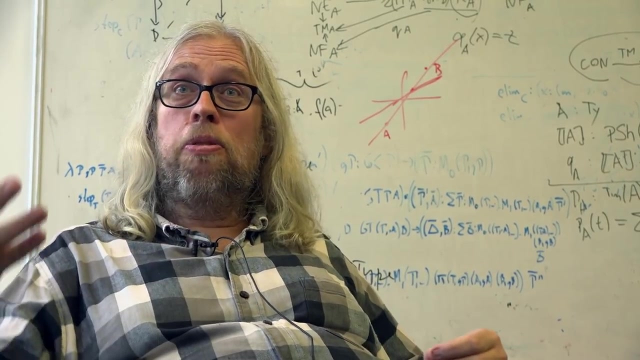 in various ways. So, for example, in the standard encoding, in set theory, there's a very strange artifact. For example, one number is an element of a bigger number. So if you think of natural numbers, counting numbers, it's true that two is an element of three. 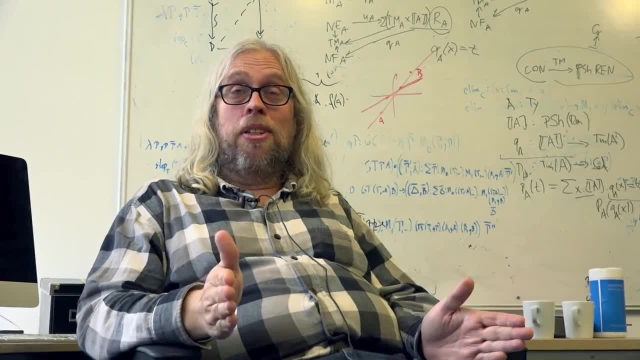 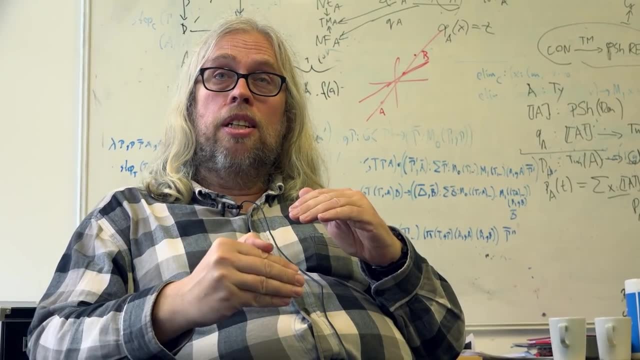 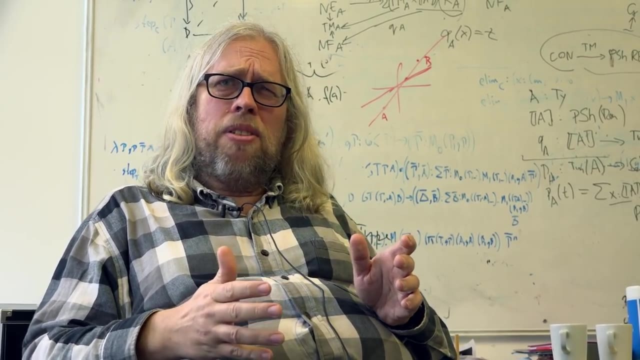 Doesn't really make any sense, right? It's just the way it's set up, Which means when you work in set theory, you can see the implementation details, how numbers are actually represented using curly brackets, And that's something which doesn't really matter. 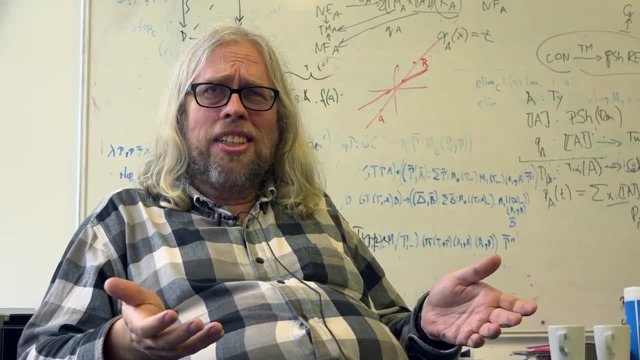 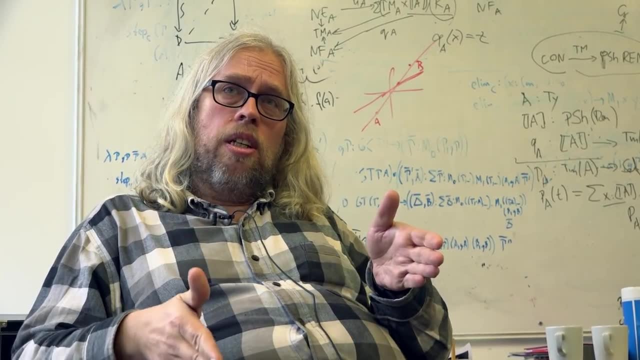 when you think about numbers, That something two is an element of three is silly, yeah, But you can't hide this In type theory. when you introduce natural numbers in type theory, you cannot talk about numbers in encoding how they're actually represented. 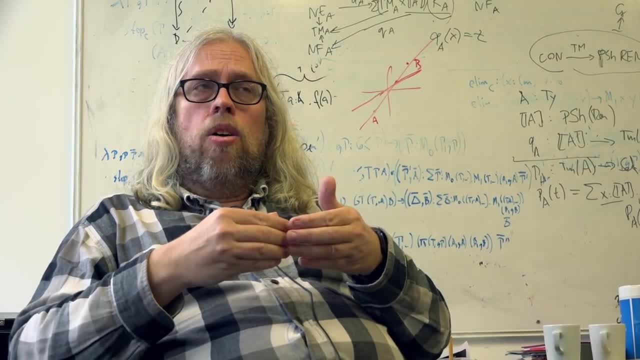 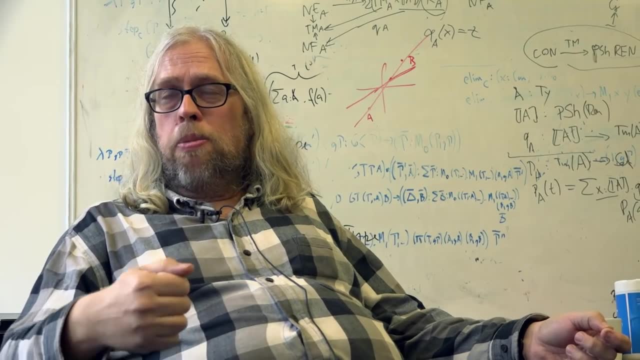 So, for example, numbers are often represented following an idea of an Italian mathematician called Peano. He said: zero is a natural number, and if you have a natural number, then the number plus one is also natural numbers. And that's the way. 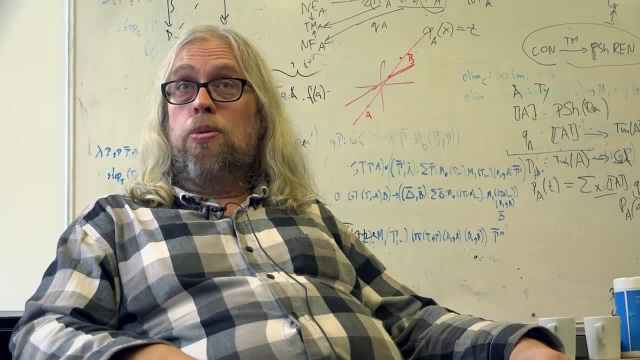 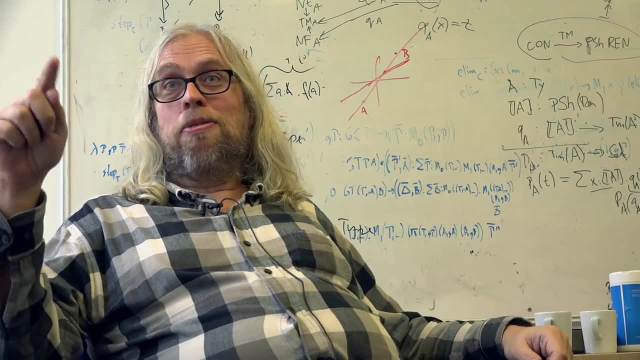 we can build all natural numbers, But there are other ways to do this, right. So this is a very. when you write numbers in the system, they become very long, right, Because you write plus one, plus one, plus one. 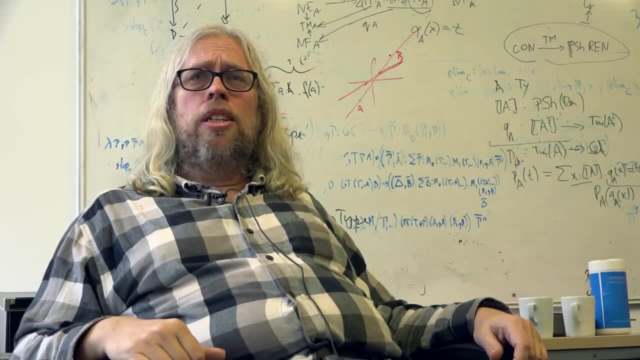 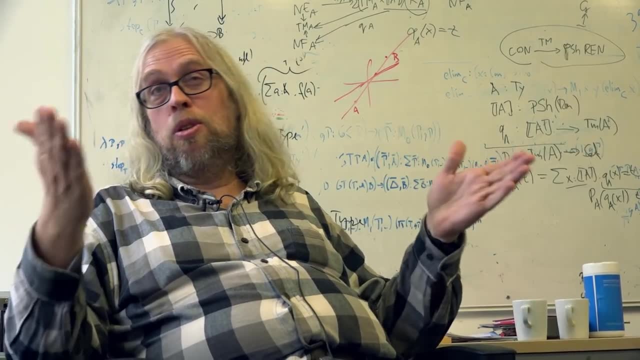 so that's not a very good system. So what we rather like to do is using binary encoding of numbers, using zero and one. That's much shorter- I mean, it's still longer than decimal, but it's much shorter than this- plus one, plus one, plus one. 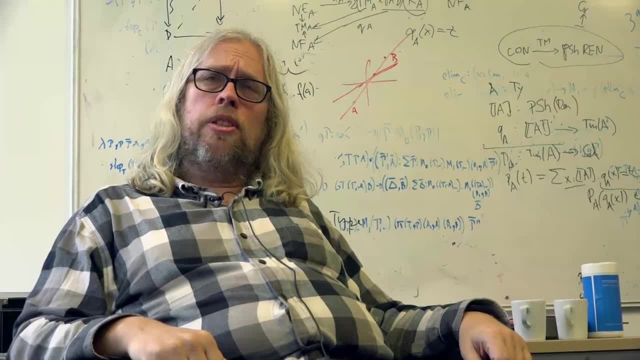 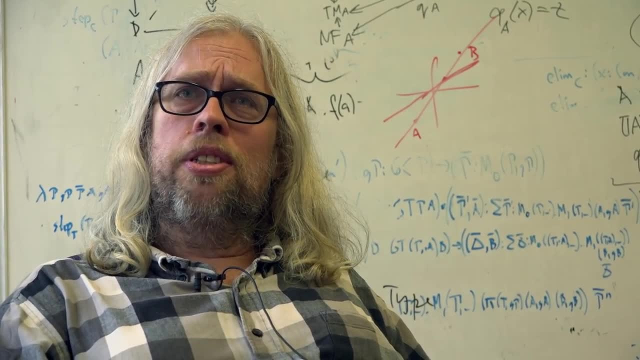 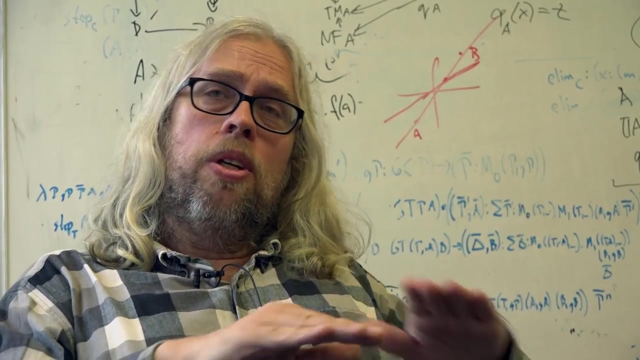 And these are two ways of encoding the natural numbers. Now, in type theory, you cannot express a difference between these two encodings because they are actually in a way the same. They're just, they exhibit the same concept. So you automatically hide implementation details. 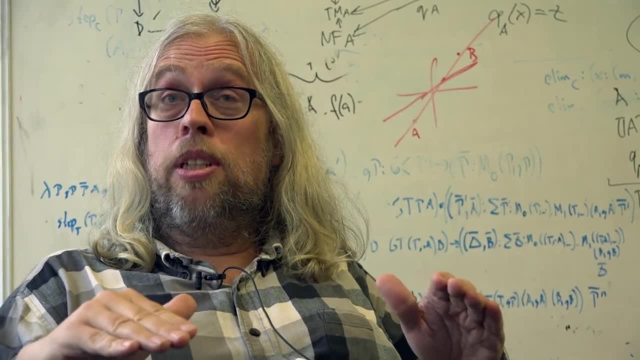 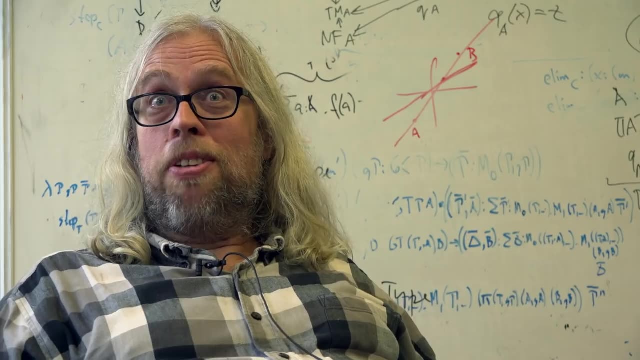 Like: that's what we want to do in computer science. We want to hide implementation details because, like, if you want to change one implementation for another, you don't want to go all up. everything which uses this has to be rewritten. 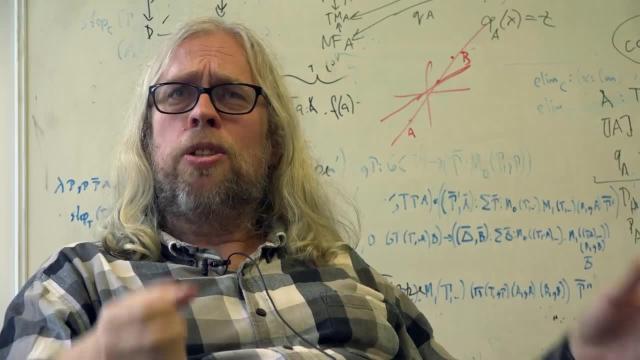 You want to say, okay, I'll just plug something else in and it works. yeah, So you want to be able to plug in when you use the piano numbers and it gets too cumbersome and I don't want it to plug in my binary numbers. 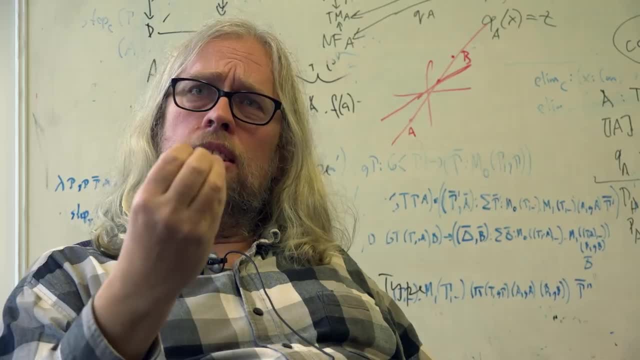 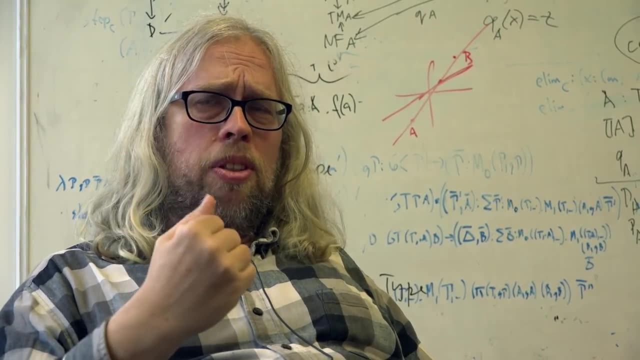 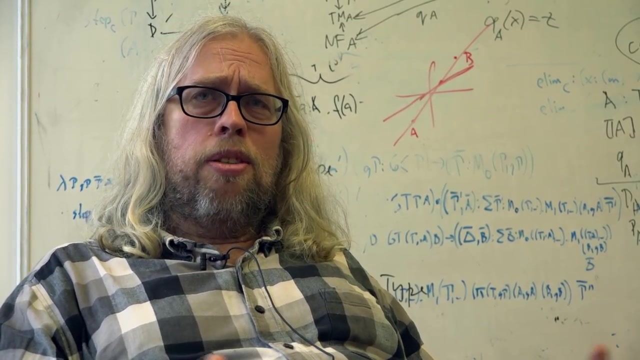 and nothing should change. And that's how type theory is designed. And from this homotopy type theory comes a very important principle which is called the univalence principle, And it basically says the two things which are equivalent, like the binary numbers and the unary numbers. 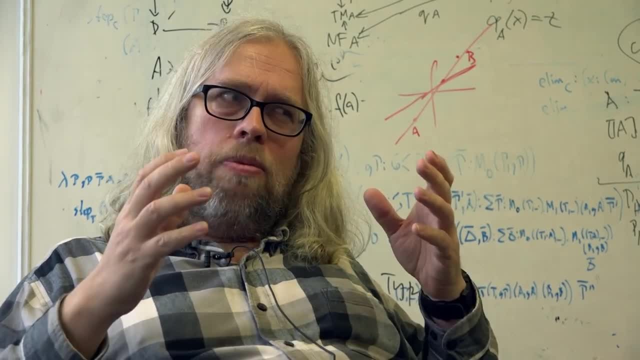 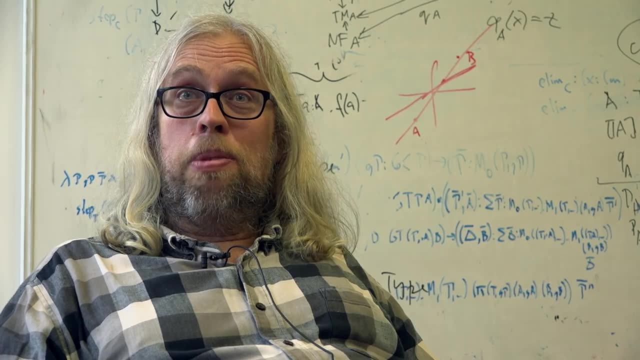 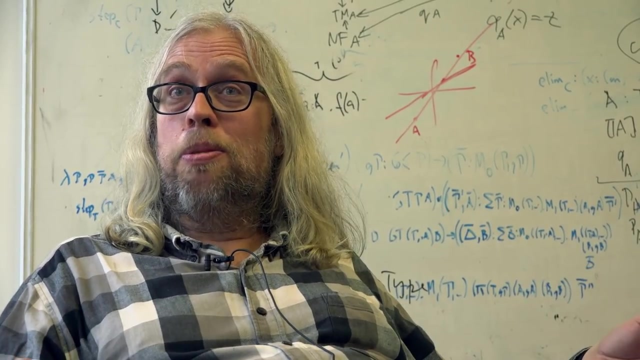 the piano numbers, then they are equal. We cannot, not just we cannot talk about implementation details, but because we cannot talk about implementation details, two things which behave the same from outside are actually considered to be the same. Is this changing massively? 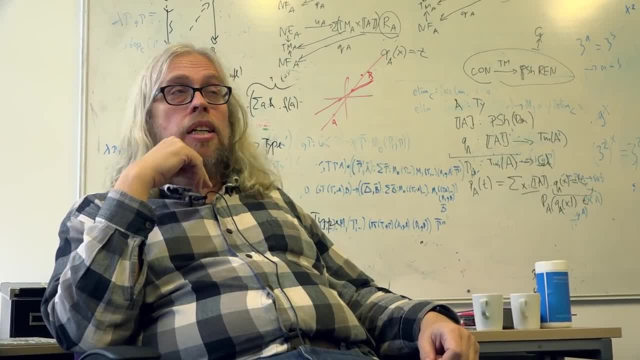 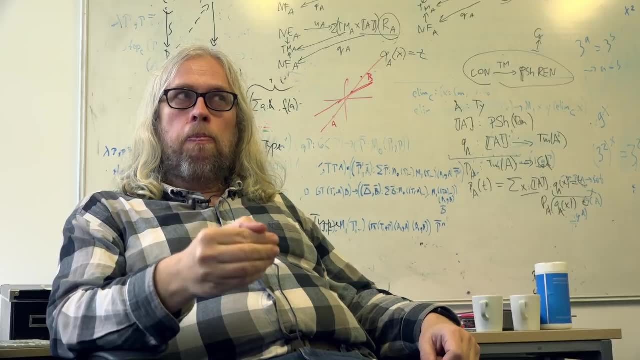 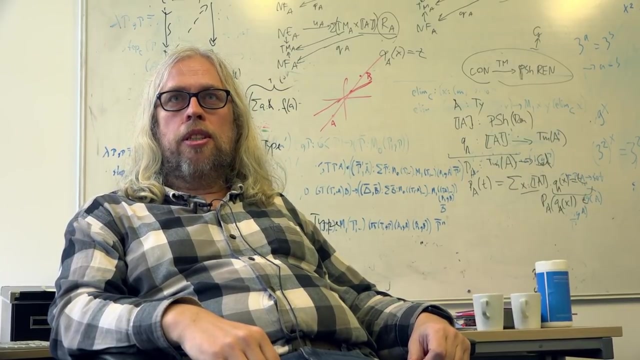 the way people think about things in other areas, then Yes, Let's say it has the potential of doing this. yeah, So homotopy type theory has been suggested as a new foundation of mathematics. Yeah, people can just move into it. 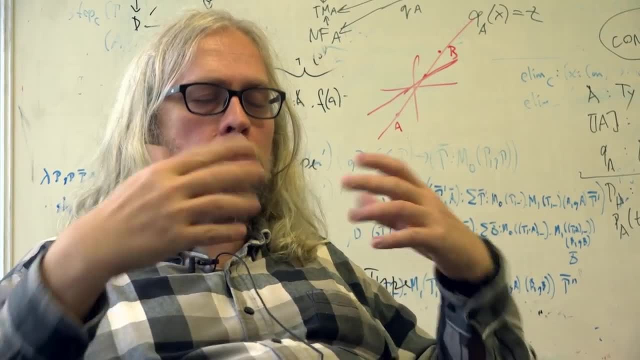 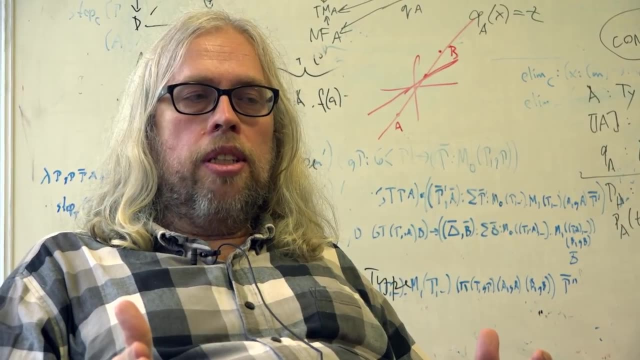 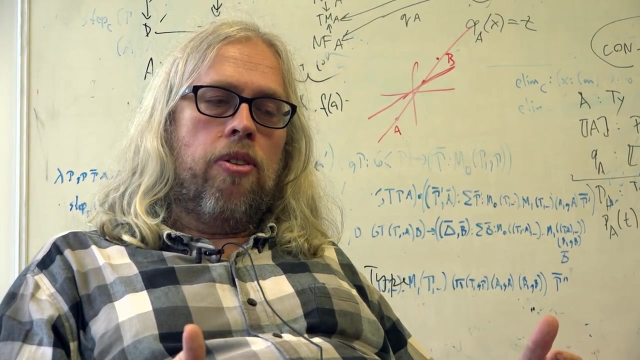 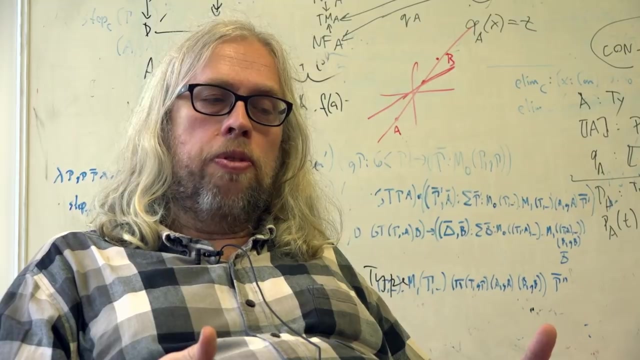 They can learn logical reasoning and abstract mathematics just coming from this programming angle. yeah, So I think there is an exciting opportunity And I think, looking back to set theory, we have these new tools of proof assistance to do interactive proofs And, in a way, it would be a shame. 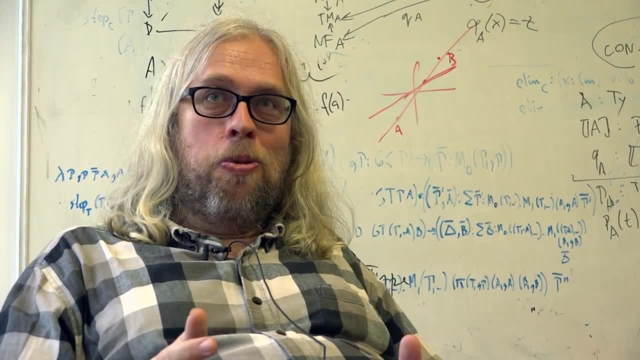 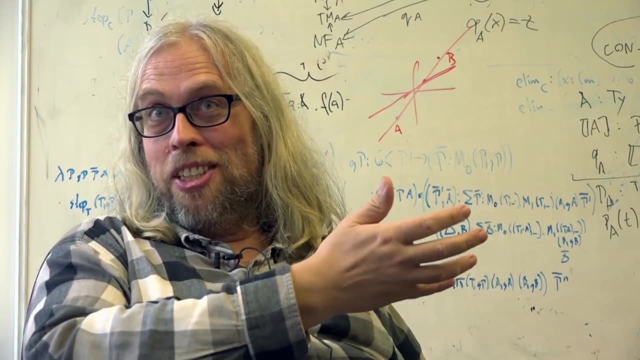 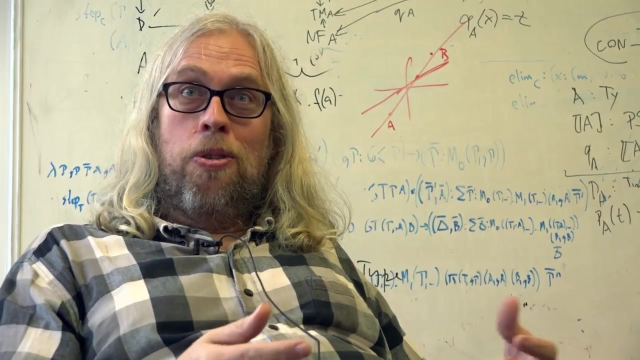 if we use this new technology to formalize the mathematics from the 20s and 30s, the mathematics of, let's say, yesterday, yeah, But there is an exciting new opportunity here to use, to really use new mathematical ideas.